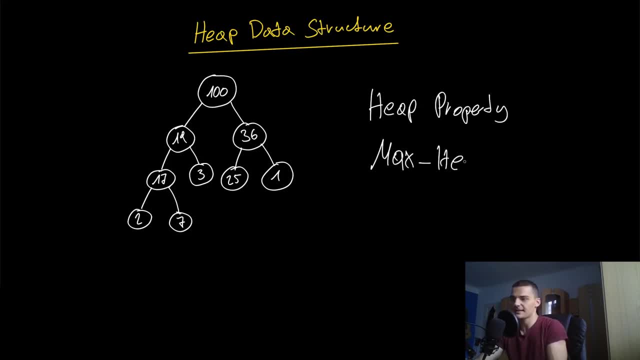 we're looking at a max heap and this means that every child has to be smaller than its parent. So each parent node has to be larger than all of its childs. So 17 is larger than 2 and 7, 19 is larger. 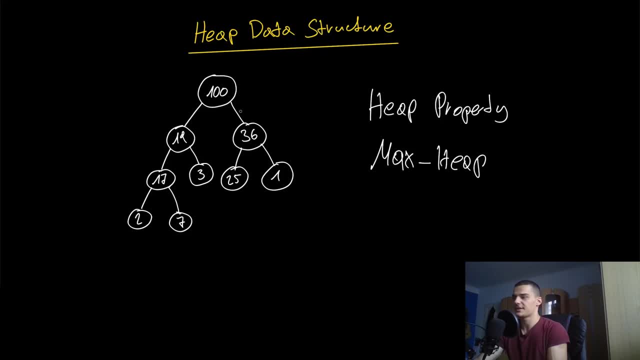 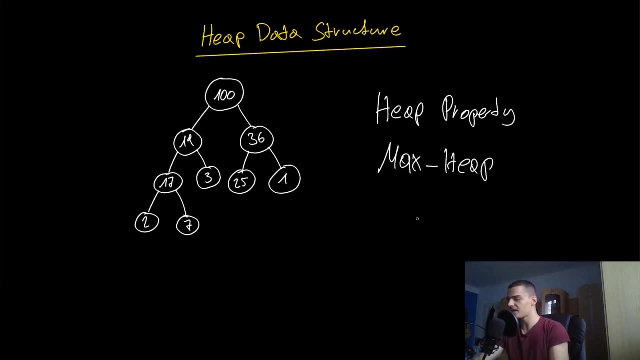 than 17 and 3,. 100 is larger than 19 and 36.. 36 is larger than 25 and 1.. So in this case, the heap property of a max heap is fulfilled. This is essentially what you always want to maintain in a heap. You also have the min heap. 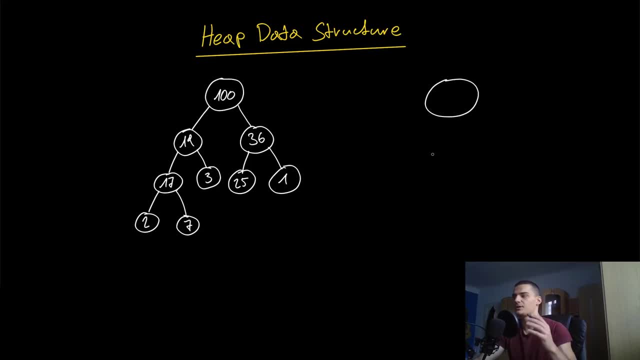 for example, where it's the other way around. So the heap property here is that the parent is always smaller than its children. So you could have something like 5, and then you have 16 and 28.. Well, that's not an 8, 28.. And then, here you have something even larger. 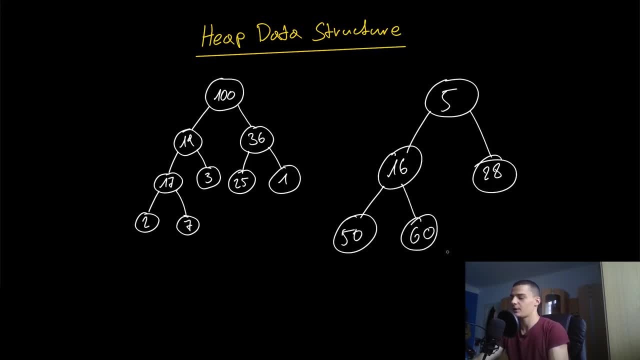 So 50 and 60, for example, whatever. But notice that, unlike a data structure, we're going to learn in the future, or learn about in the future, the binary search tree. it doesn't matter if the left node is larger than the right node or the left node is. you know, there's no specific order. The 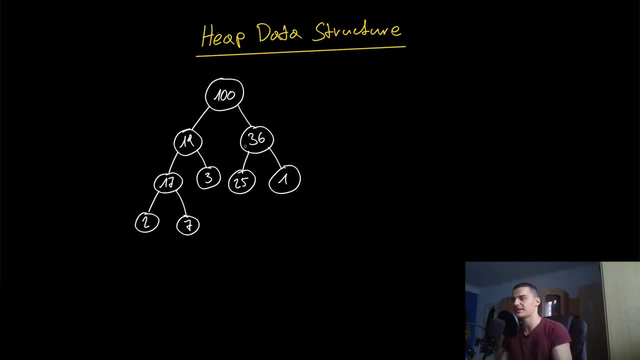 only thing that you want is that the parent is always larger than its children. This is in the max heap at least, or the other way around in the min heap. We don't care about the left child being larger or smaller than the right child. The only thing we want is that this is. 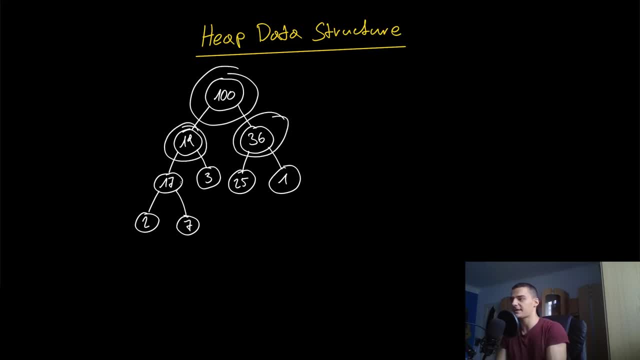 the largest element, then these are the two largest elements after that, and so on. So this is the basic heap property in a max heap and in the min heap it's the other way around. Now let us go back to the idea of a priority queue. What we wanted out of a priority queue is that elements get processed. 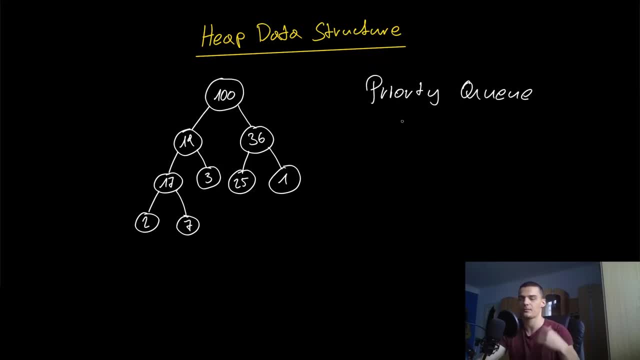 based on their priorities. So we had a bunch of elements and they had a priority of one, two, three, four, five, ten, a thousand, whatever, And we can say the lowest number means the highest priority or the largest number means it's the highest priority. 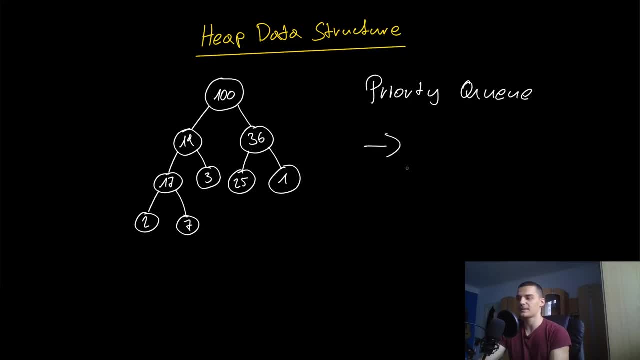 And then what we wanted to do is we want to enqueue elements. They get sorted into the list in logarithmic time. This was our goal, and we also wanted to dequeue the element with the highest priority first. Now we talked about how we could do that with a linked list, but the sorting and 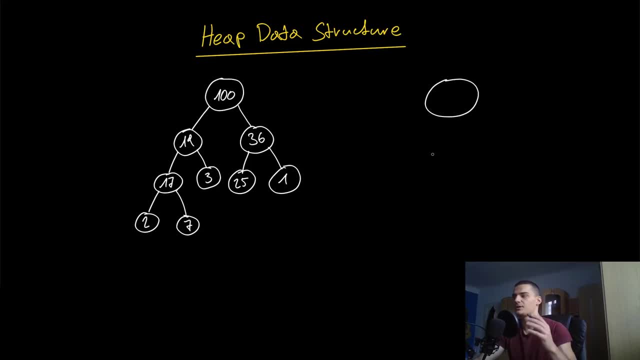 for example, where it's the other way around. So the heap property here is that the parent is always smaller than its children. So you could have something like 5, and then you have 16 and 28.. Well, that's not an 8, 28.. And then, here you have something even larger. 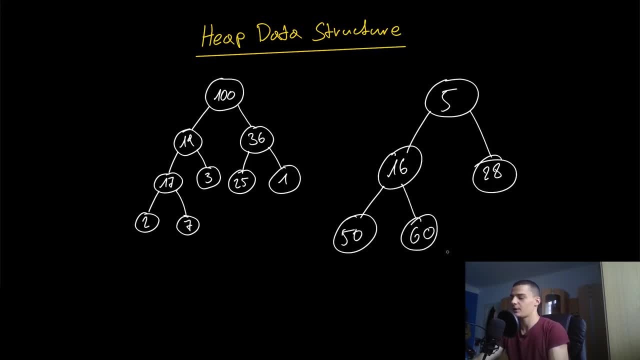 So 50 and 60, for example, whatever. But notice that, unlike a data structure, we're going to learn in the future, or learn about in the future, the binary search tree. it doesn't matter if the left node is larger than the right node or the left node is. you know, there's no specific order. The 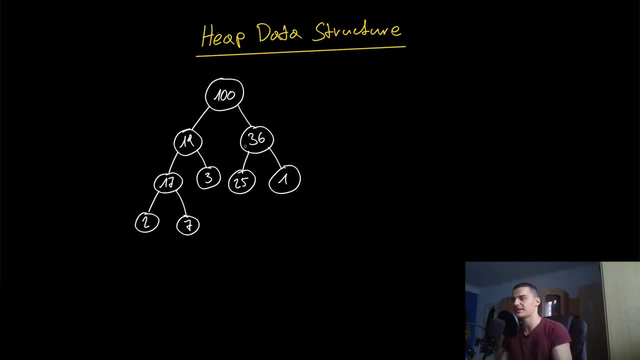 only thing that you want is that the parent is always larger than its children. This is in the max heap at least, or the other way around in the min heap. We don't care about the left child being larger or smaller than the right child. The only thing we want is that this is. 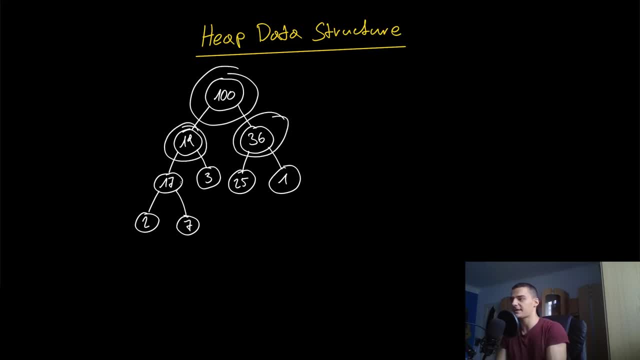 the largest element, then these are the two largest elements after that, and so on. So this is the basic heap property in a max heap and in the min heap it's the other way around. Now let us go back to the idea of a priority queue. What we wanted out of a priority queue is that elements get processed. 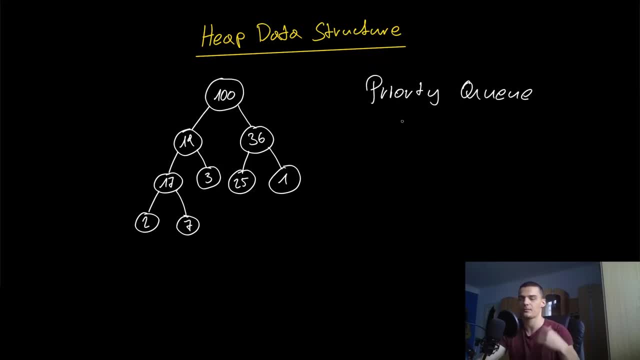 based on their priorities. So we had a bunch of elements and they had a priority of one, two, three, four, five, ten, a thousand, whatever, And we can say the lowest number means the highest priority or the largest number means it's the highest priority. 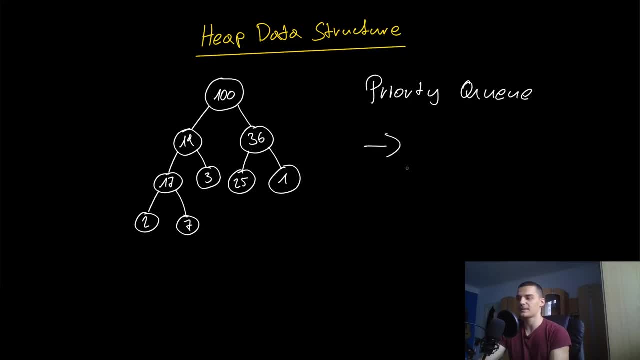 And then what we wanted to do is we want to enqueue elements. They get sorted into the list in logarithmic time. This was our goal, and we also wanted to dequeue the element with the highest priority first. Now we talked about how we could do that with a linked list, but the sorting and 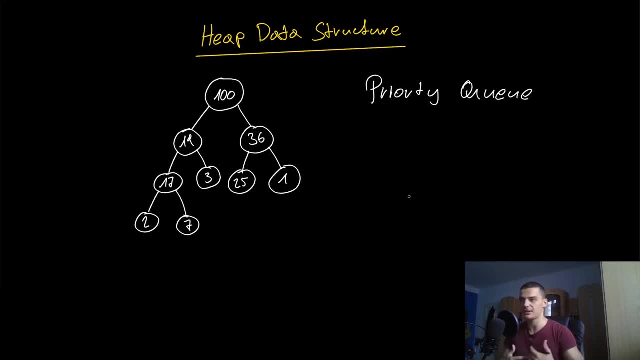 the accessing would only be done in linear time or, possible, in linear or pseudo-linear time. So what we need to do is- or what we wanted to do is we want to find a logarithmic way. Now let's go to our heap here and look at it. Now, what we have to 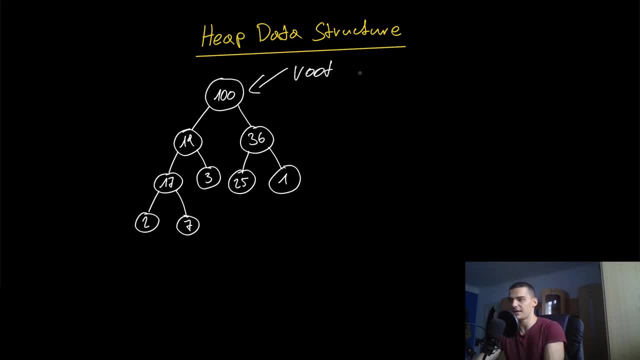 here at the root in a max heap is always the largest element and the root node can be accessed in constant time since it's always the same address. If you think about this tree as having all these childs, all these positions in fixed memory addresses, you can say that the root 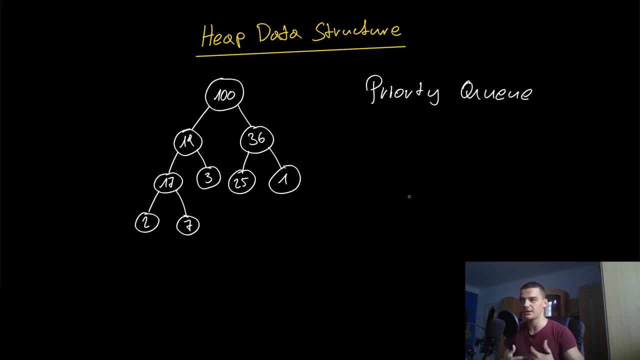 the accessing would only be done in linear time or, possible, in linear or pseudo-linear time. So what we need to do is- or what we wanted to do is, we want to find a logarithmic way. Now let's go to our heap here and look at it. Now, what we have. 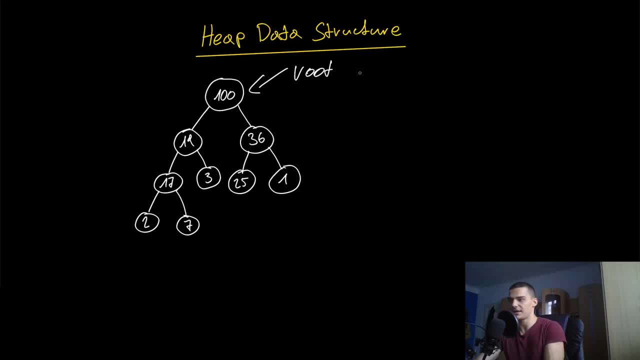 here at the root in a max heap is always the largest element and the root node can be accessed in constant time since it's always the same address. If you think about this tree as having all these childs, all these positions in fixed memory addresses, you can say that the 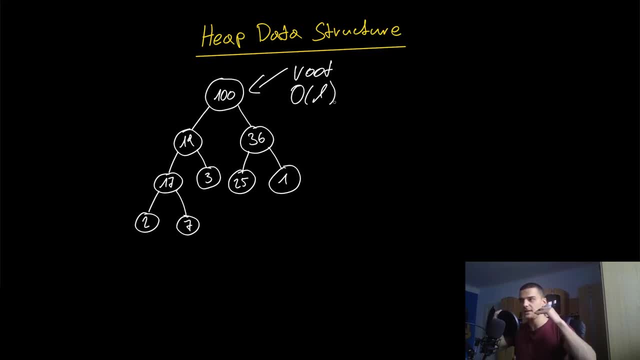 root node is always the largest element. If the heap property is satisfied, the root node will always be the largest element. And if we say that the largest element is the largest priority, the highest priority, we can say that the element that has to be dequeued next. 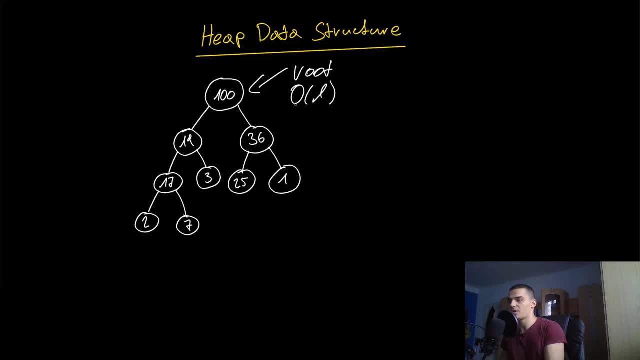 is always at the root node, So in this case we could always just pop this out, basically, and we could process the root node. Now, this would be deleting an element, and we're going to talk about that in a second how this would work and why this is possible in logarithmic time. 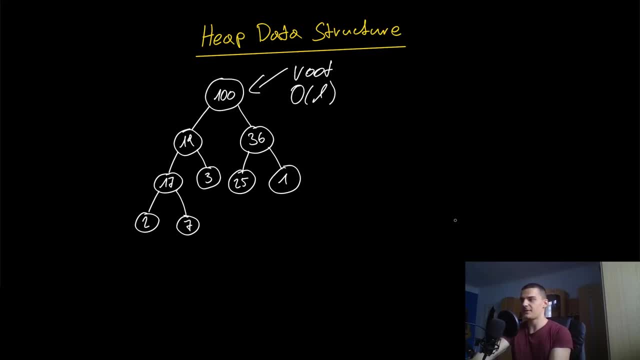 But let's talk about inserting first, because in this case it's very easy to see that the root element is always going to be the largest one, but this part down here doesn't look really sorted. We have 19,, 36,, 3,, 1, 2, all over the place. 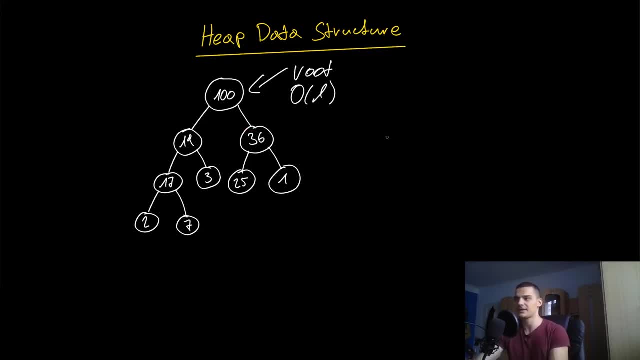 So let's think about how we can insert elements into this heap data structure in logarithmic time without violating the heap property. Now, what we would do for that is, we would just go ahead and append the new element at the end of this heap data structure, At the end. 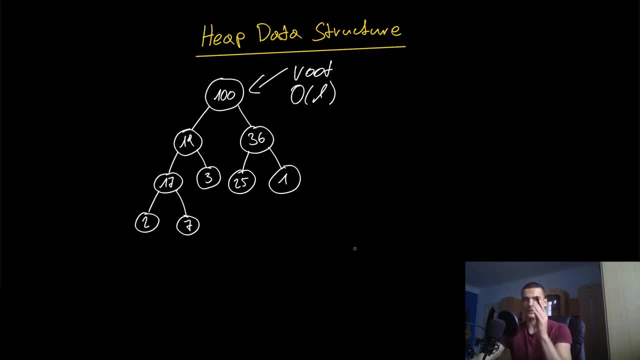 means that we fill this tree data structure up from left to right. We don't just add it somewhere here, but the next element, whatever it is, will be the left child of this, the next free place. If you look at it like that, this is the first position. then we have, you know. 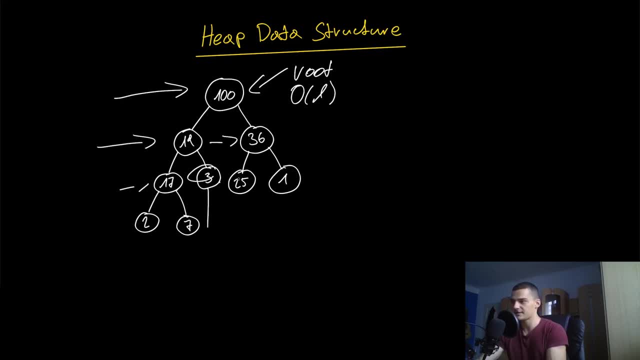 2,, 3,, 4,, 5,, 6,, 7,, 8,, 9 and so on. These are the positions, so this would be the next one. that's free. So whatever element we add here, let's say we add the number. 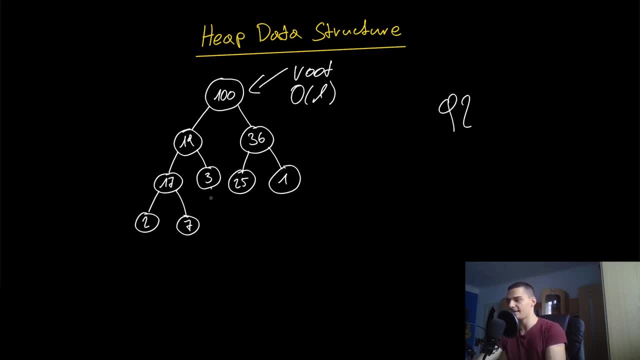 92 here. whenever we add a new element, we just append it onto the next free position here. So what we do is we say, okay, this is 92 here and the problem is now the heap property is violated, So what we do in order to restore it? 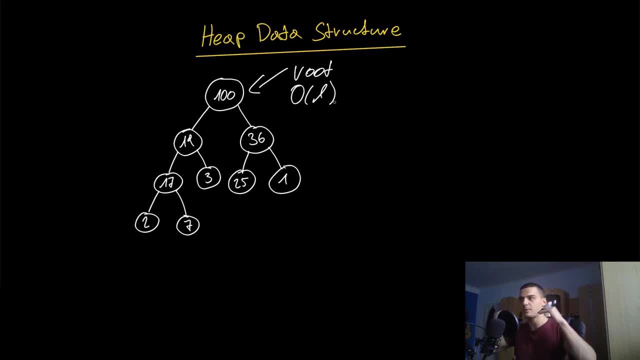 node is always the largest element. If the heap property is satisfied, the root node will always be the largest element. And if we say that the largest element is the largest priority, the highest priority, we can say that the element that has to be dequeued next is: 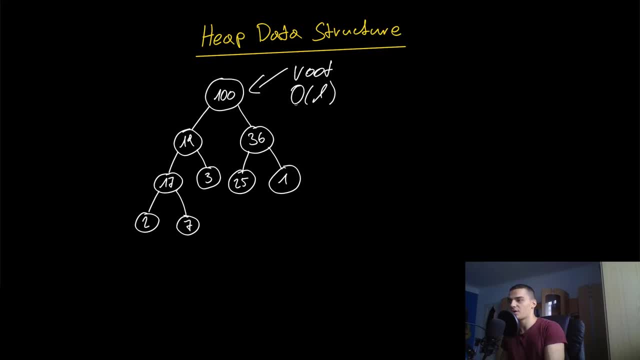 always at the root node. So in this case we could always just pop this out, basically, and we could process the root node. Now, this would be deleting an element, and we're going to talk about that in a second, how this would work and why this is possible in logarithmic time. But let's talk. 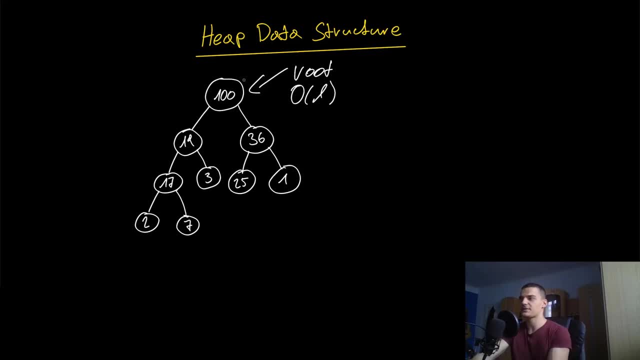 about inserting first, because in this case it's very easy to see that the root element is always going to be the largest one. but this part down here doesn't look really sorted. We have 19,, 36,, 3,, 1,, 2, all over the place. 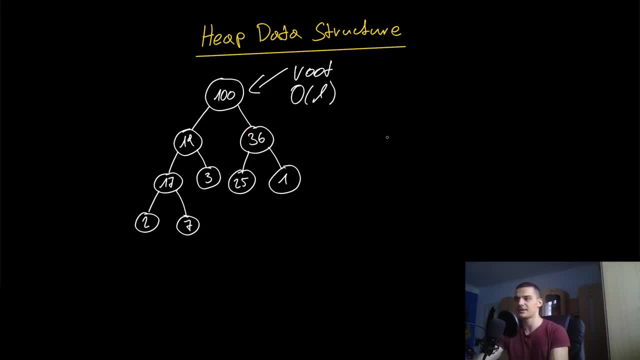 So let's think about how we can insert elements into this heap data structure in logarithmic time without violating the heap property. Now, what we would do for that is, we would just go ahead and append the new element at the end of this heap data structure And at 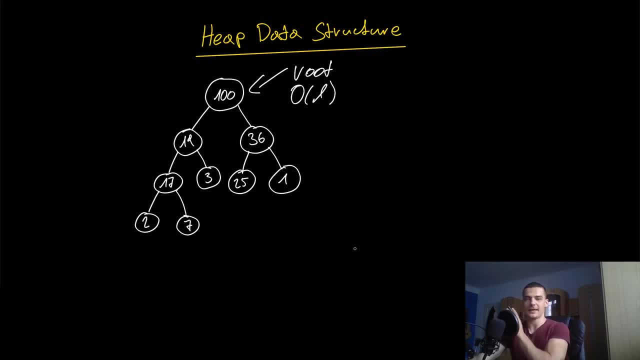 the end means that we fill this tree data structure up from left to right. We don't just add it somewhere here, but the next element, whatever it is, will be the left child of this, the next free place. If you look at it like that, this is the first position, then we have. 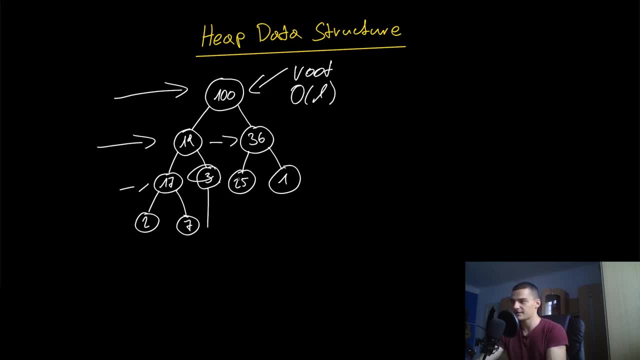 2,, 3,, 4,, 5,, 6,, 7,, 8,, 9 and so on. These are the positions, So this would be the next one that's free. So whatever element we add here, let's say, we add the number 92 here whenever we add a new. 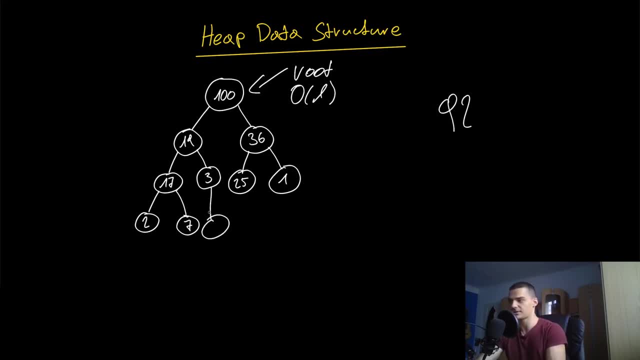 element, we just append it onto the next free position here. So what we do is we say: okay, this is 92 here, and the problem is now the heap property is violated. So what we do in order to restore it, in order to satisfy it again, is we perform a so-called heapify up operation. Heapify up, Which? 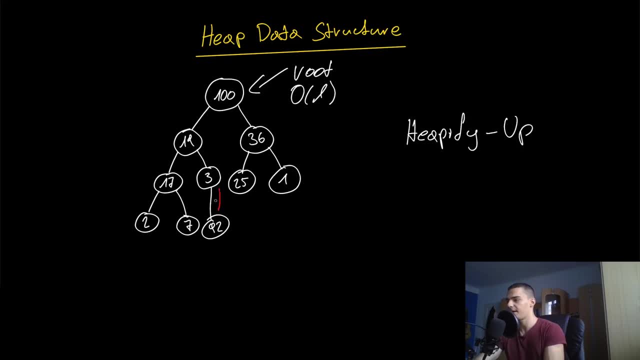 essentially means that we just go to this element here and compare it to its parent. So we say, okay, 3 is less than 92. That violates the heap property. So what I'm going to do is I'm going to change it by swapping these two nodes. Now let me delete them real quick. So we're swapping 92 and 3.. 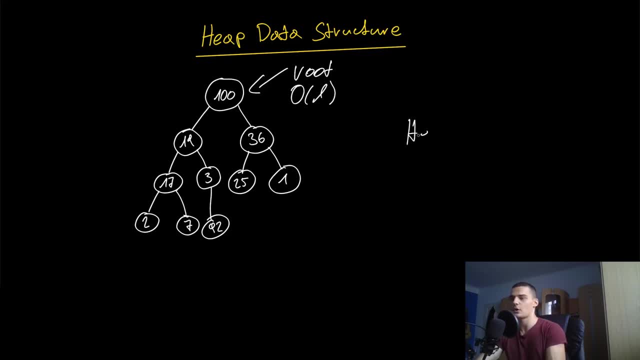 in order to satisfy it again is we perform a so-called heapify up operation. heapify up, which essentially means that we just go to this element here and compare it to its parent. So we say, okay, 3 is less than 92, that violates the heap property. so what I'm going to do is: 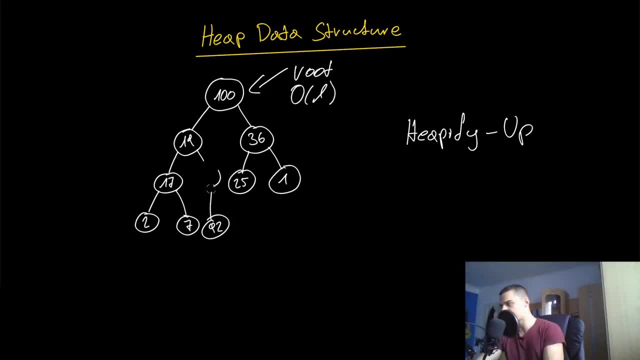 I'm going to change it by swapping these two nodes. Now let me delete them real quick. So we're swapping 92 and 3.. So we have 92 here and 3 is the left child of 92, and what we have now is we have the next check, because now what we 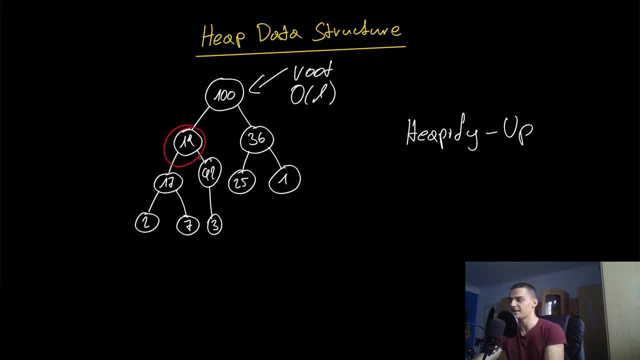 have to do is we have to compare it to its parent again. We can see 19 is less than 92.. So what we do is we perform another swap here and we swap 92 with 19.. 92 and 19.. So we have 92 here and 19 here. By the way, we don't need to check for that 17 because since 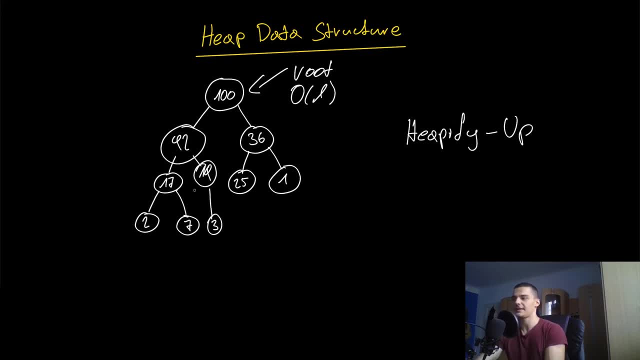 92 was already larger than 19 and 19 was the parent of 17 and thus larger than 17,. we don't need to compare 92 to 17. it's going to be automatically larger than 17.. Now what we have to do is we have to compare it to 100, but 100 is larger than. 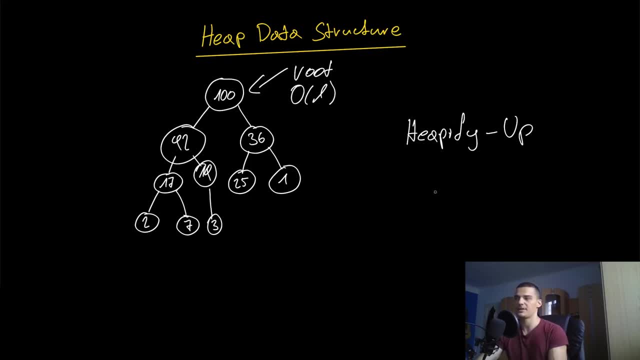 a 92. So it's done and we have the heap properties satisfied again. Now this is possible, obviously, in logarithmic time, because again we have this, the same thing that we have with Merge, Sort and all that. We have the amount of levels, So we have 1, 2, 3 full levels. 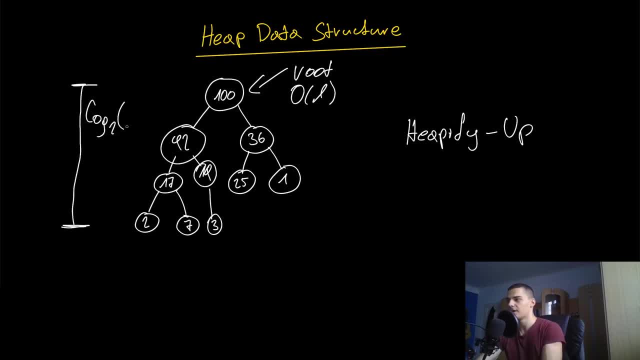 and the amount of levels is the logarithm of base two of the amount of elements. so the amount of levels, levels is logarithmic based on the amount of elements and uh, because we don't need to compare more than the amount or more times than the amount of levels we have to uh to do the 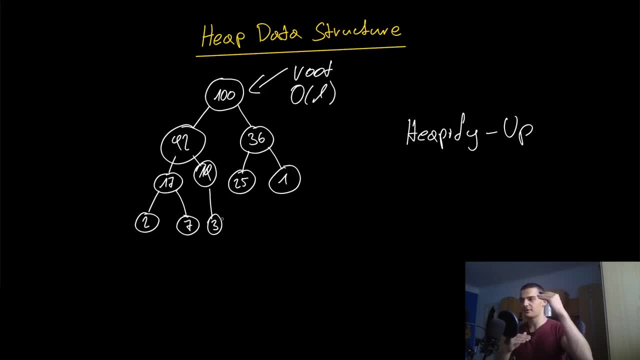 comparisons a maximum amount of time, as there are levels. well, this was not an english sentence. what what we need to do is we need to start at the bottom and, in the worst case, we need to compare to all the elements through all these levels, to all its parents, essentially, until we get to the 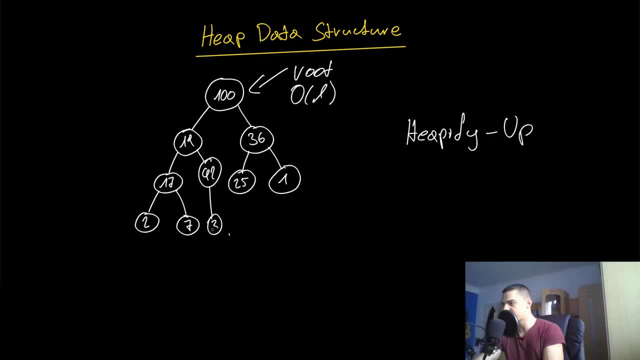 So we have 92 here and 3 is the left child of 92. And what we have now is we have the next check, Because now what we have to do is we have to compare it to its parent again. We can see 19 is less than 92.. 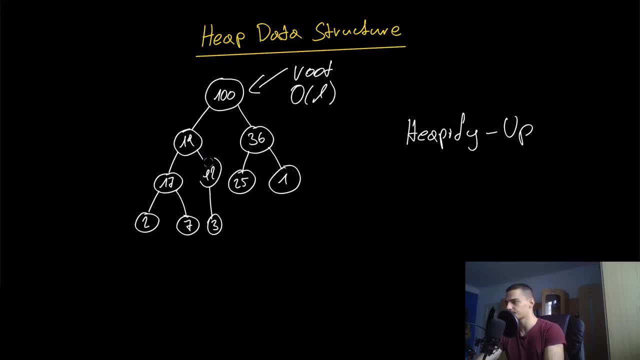 So what we do is we perform another swap here and we swap 92 with 19.. 92 and 19.. So we have 92 here and 19 here. By the way, we don't need to check for that 17, because 92 is already larger than 19 and 19 was a parent of 17 and 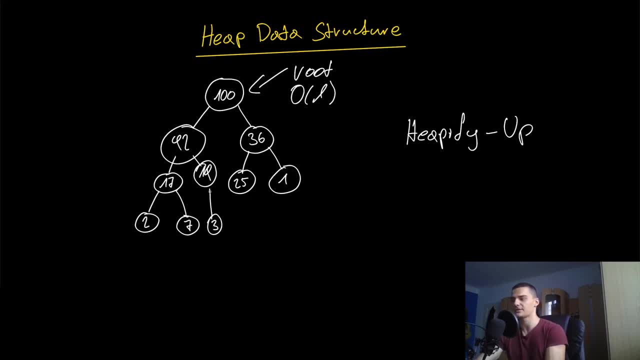 that's larger than 17.. We don't need to compare 92 to 17.. It's going to be automatically larger than 17.. Now what we have to do is we have to compare it to 100, but 100 is larger than. 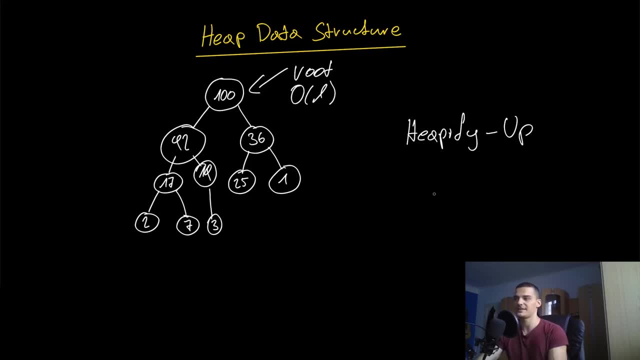 92. So it's done and we have the heap properties satisfied again. Now this is possible, obviously, in logarithmic time, because again we have this, the same thing that we have with merge, sort and all that. We have the amount of levels, So we have 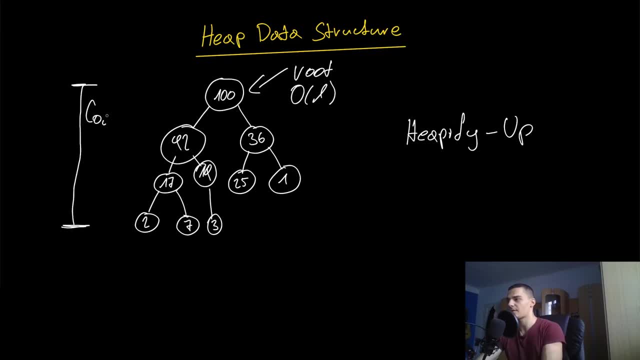 one, two, three, four levels and the amount of levels is the logarithm of base two of the amount of elements. so the amount of levels, levels is logarithmic based on the amount of elements and because we don't need to compare more than the amount or more times than the amount of levels, we 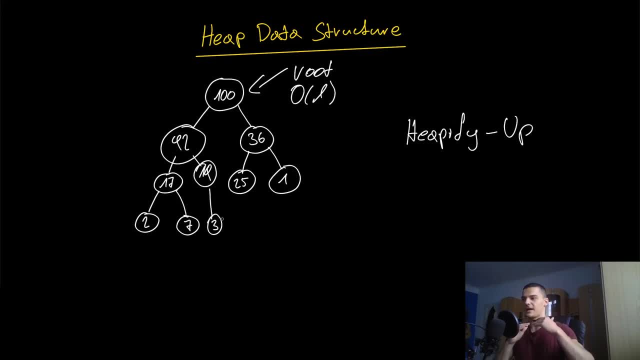 have to to do the comparisons a maximum amount of time, as there are levels. well, this was not an english sentence. what what we need to do is we need to start at the bottom and, in the worst case, we need to compare to all the elements through all these levels, to all its parents, essentially. 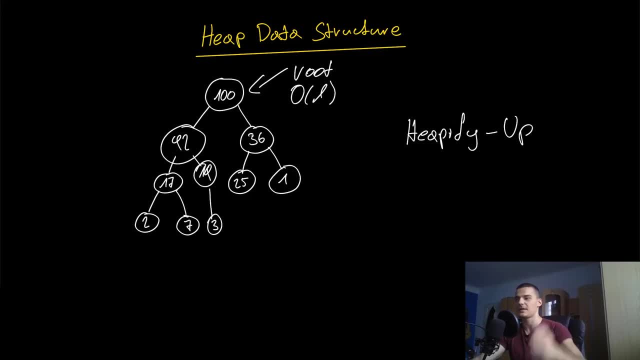 until we get to the root node. so the worst case is we go through all the levels, but the amount of levels is logarithmic. the comparison itself is constant. thus the process of inserting or inserting is logarithmic as well. so heapify up and inserting are a logarithmic operation. so now we know how to. 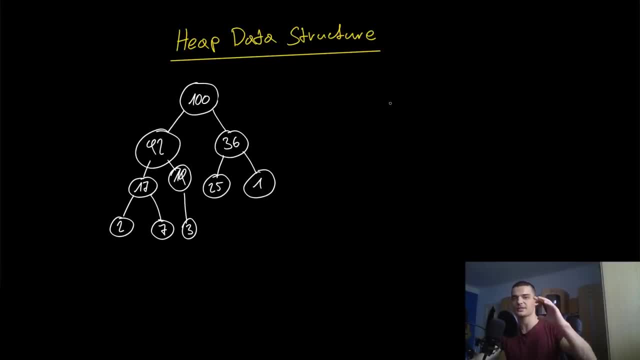 enqueue elements in logarithmic time. we know how to put new elements into this heap data structure, into this priority queue, but we also need to find a way to pop out the elements, to process the elements, because we already set 100 here or the root node is always going to be the next element to be processed. 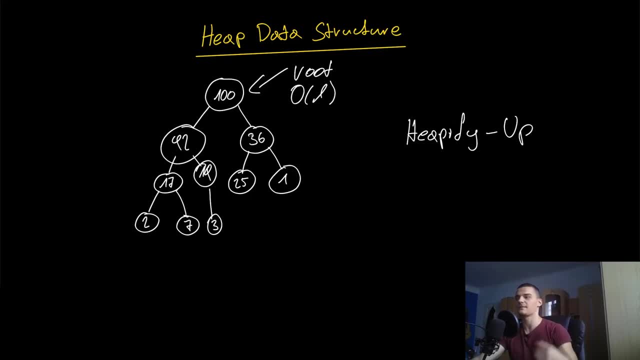 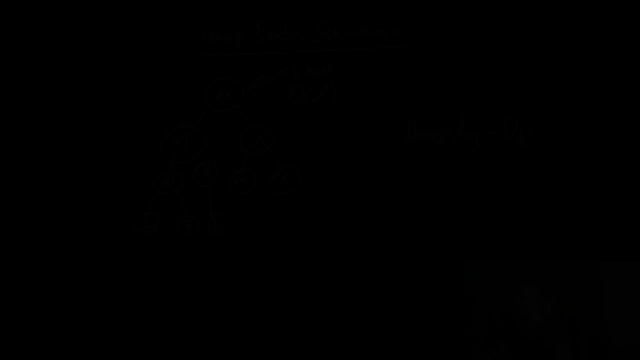 root node. so the worst case is, we go through all the levels, but the amount of levels is logarithmic. the comparison itself is constant. thus the process of inserting, or inserting is logarithmic as well. so heapify up and inserting are a logarithmic operation. so now we know how to enqueue elements. 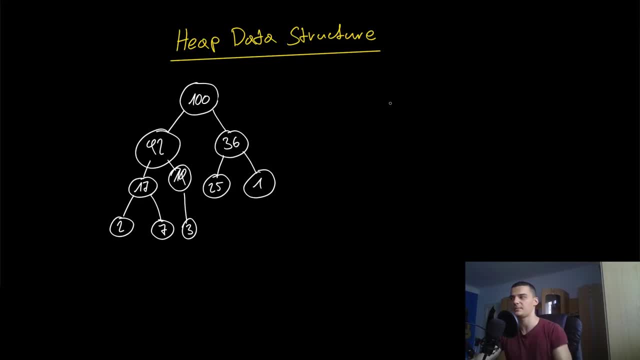 in logarithmic time. we know how to put new elements into this heap data structure, into this priority queue, but we also need to find a way to pop out the elements, to process the elements, because we already set 100 here or the root node is always going to be the next element to be processed, the highest value. 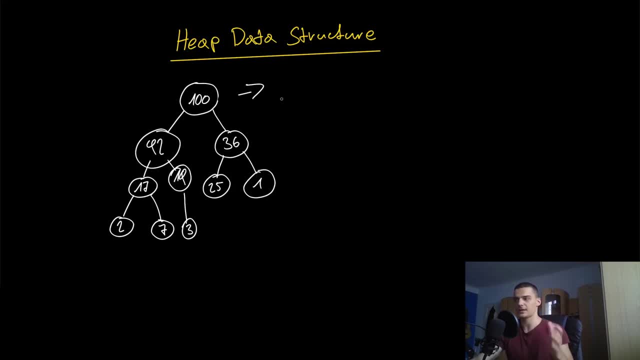 will be at the root node. in a min heap it's going to be the lowest value depending on what kind of priority you're interested in and we want to process it. but then after processing it, you know you need to remove it from the heap data structure and if we just remove 100, uh you have an empty. 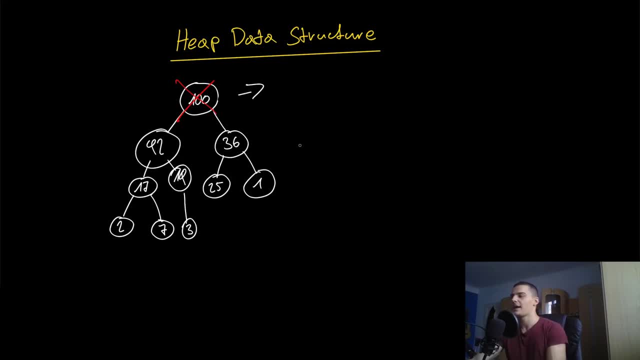 root node and no longer any tree. you don't have a tree anymore, um, and if you just shift around some of these elements, you may be violate the heap property. so we need to find a way to pop out an element and restructure the tree so that it uh fulfills the heap property again in logarithmic. 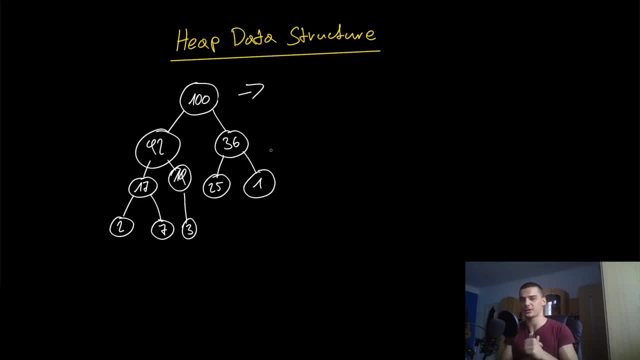 time, because then we have a method to insert an element into a data structure based on its priority in logarithmic time, and we can also pop out the largest element, so the most important element, and restructure the tree again so that it works the next time in logarithmic time as well. so 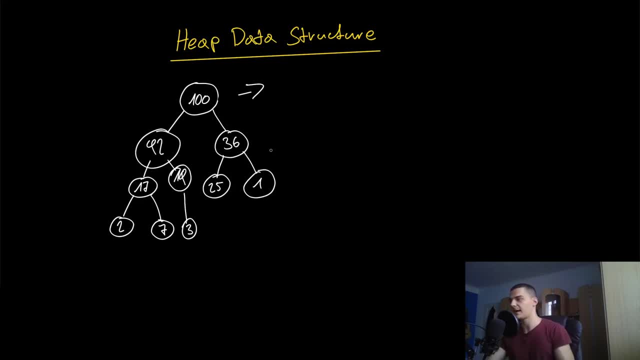 everything we want to do in the priority queue and queuing, dequeuing in logarithmic time once we figure out how to do that. so what we do here is we essentially just delete the root node and process it. so we pop it out, we say okay, 100 is the element, and then in 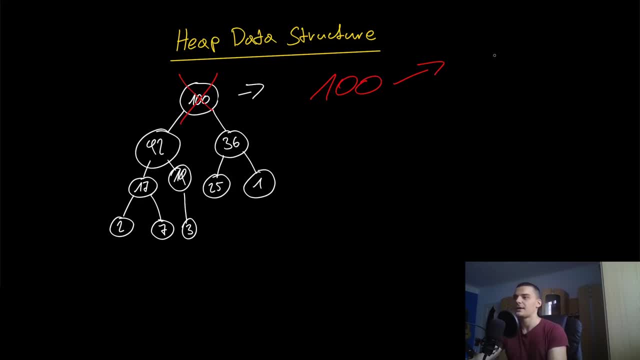 your programming code. you do whatever you want with it. you say, i don't know, do some calculations with it, but then we remove it from the tree and what we do instead, or what we do after that, is, we take the last element here. it doesn't have to be. 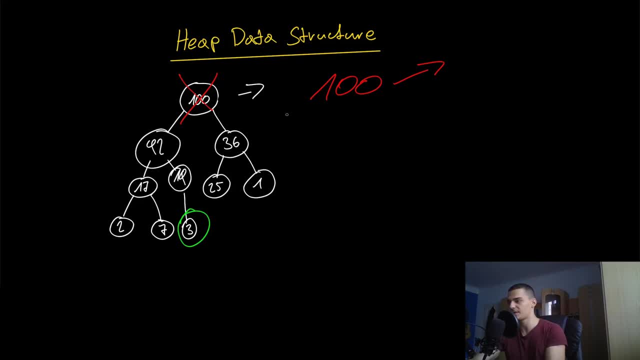 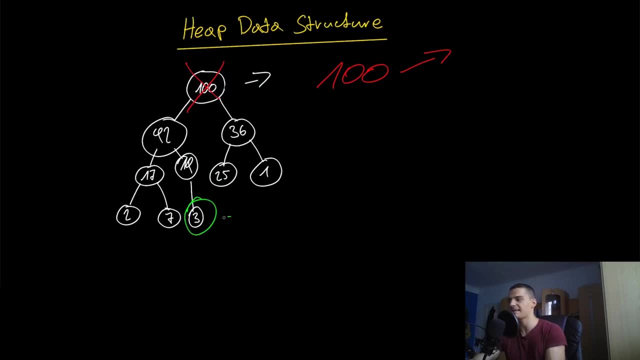 the smallest, but it's going to be the last element in the tree. we said we fill it up from left to right. so the uh, the most right element of the last level, of the last row, we take it and replace, uh, the root node, by this value. so i'm going to redraw the tree here without the circles. 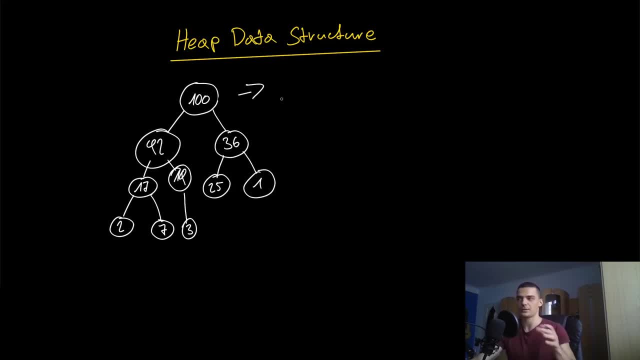 the highest value will be at the root node in a min heap. it's going to be the lowest value, depending on what kind of priority you're interested in and we want to process it. but then, after processing it, you know you need to remove it from the heap data structure and if 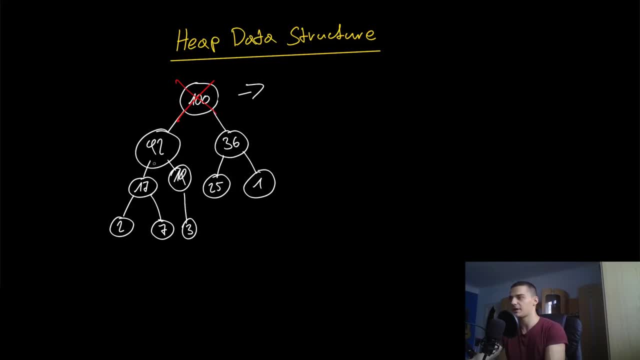 we just remove 100, you have an empty root node and no longer any tree. you don't have a tree anymore and if you just shift around the heap data structure, you're going to have an empty root node to create here. think about it. think about it. it's a dictionary term. it may need an article. 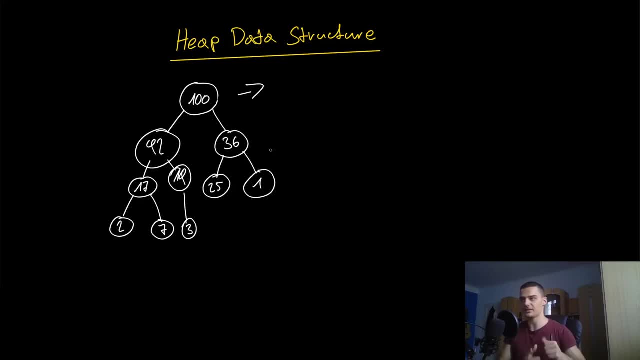 or an index or a decimal, and keep thinking about how to project an b part in a row view. another very common approach in here and our dictionary is that when a tree is happens it's already years old. since the tree is 8 months old, it's hard to understand why we. 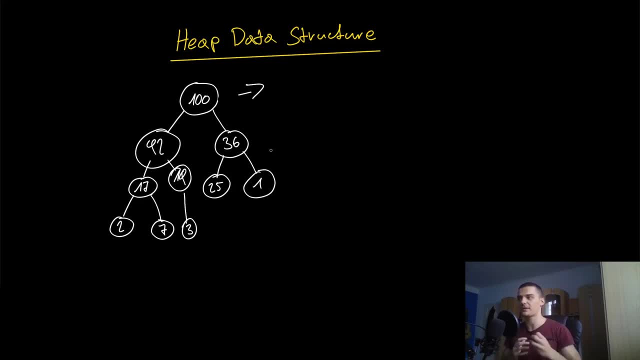 may want another size that's greater than the tree, hence theforest option. it's aersol. so another up and down sub stays to everything else. the seed starts to be the word tree. the next, and then re Android, and you name it that command, a 102 will come up in our HTML GUI. look. 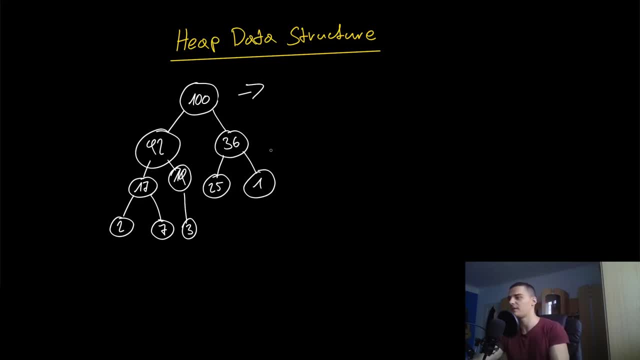 and queuing. dequeuing can be done in logarithmic time once we figure out how to do that. so what we do here is we essentially just delete the root node and process it. so we pop it out, we say okay, 100 is the element, and then in your programming code you do whatever you want with it. you say i: 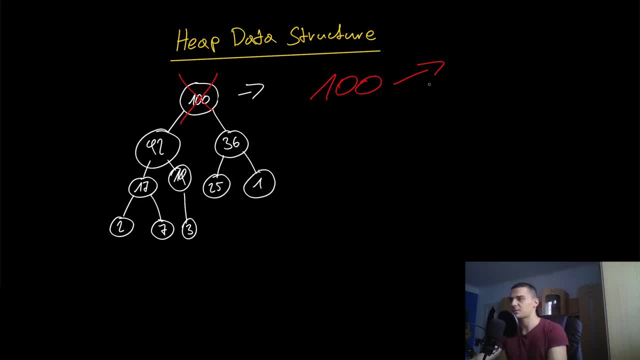 don't know, um, do some calculations with it, but then we remove it from the tree and what we do instead, or what we do after that, is we take the last element here. it doesn't have to be the smallest, but it's going to be the last element in the tree. we said we fill it up from left to right. 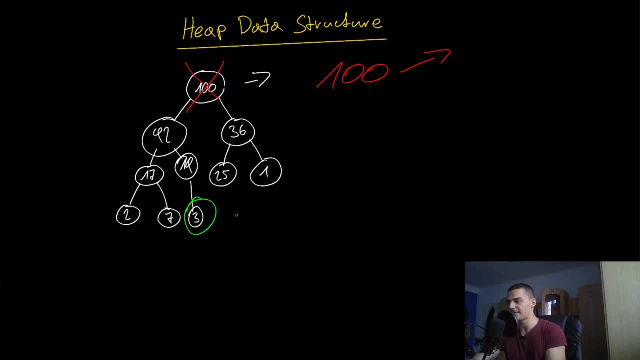 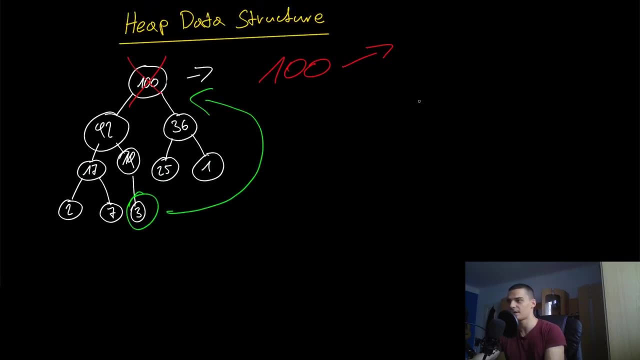 so the uh, the most right element of the last level, of the last row, we take it and replace uh, the root node, by this value. so i'm going to redraw the tree here without the circles, uh. so we have 3, 92, 36, 17, 19, 25, 1, 2 and 7. 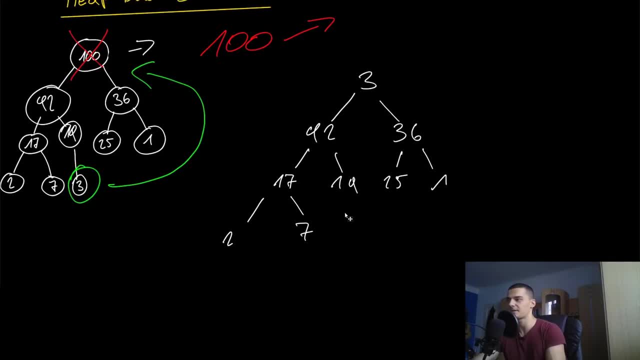 this is going to be the last element in the tree, so we take it and replace the root node by this value. this is the now, now. now the new tree, the 100, is out of the tree, and what we need to do now is: you can obviously see that the heap property is violated because there is a three, a very small. 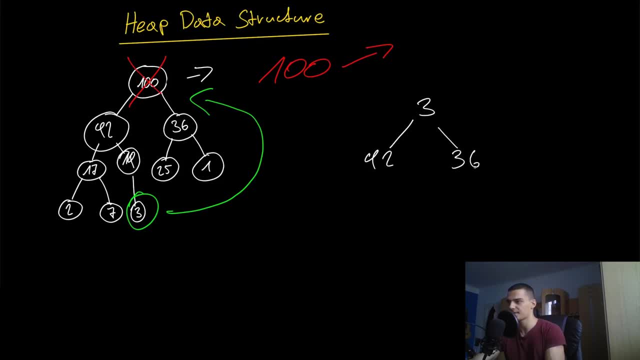 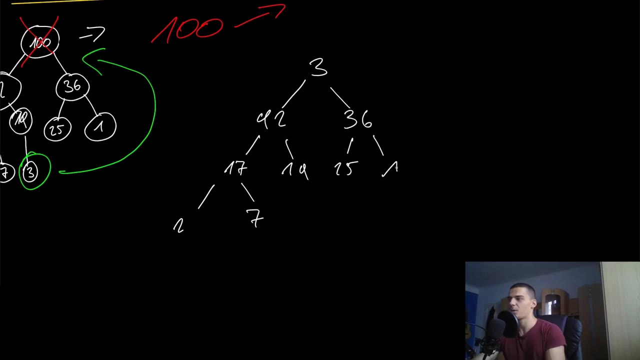 uh, so we have 3, 92, 36, 17, 19, 25, 1, 2 and 7.. this is the now. now the new tree, the 100 is out of the tree. now is you can obviously see that the heap property is violated because there is a three. 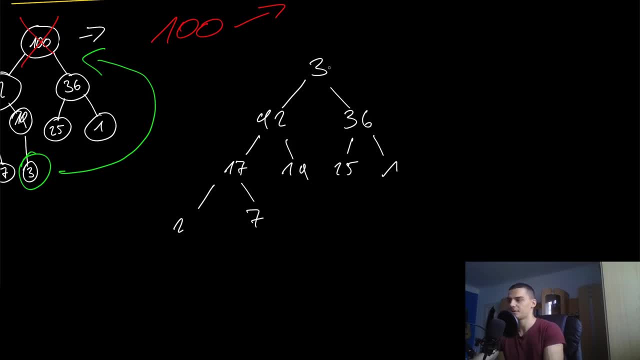 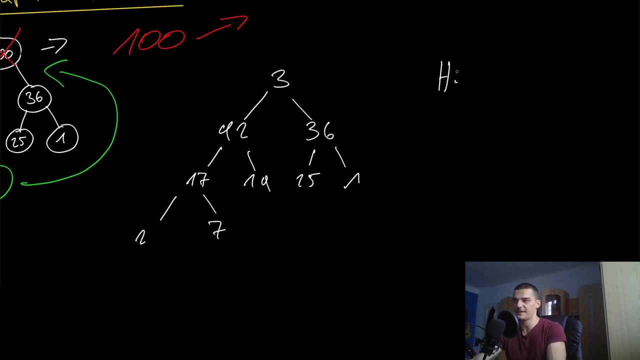 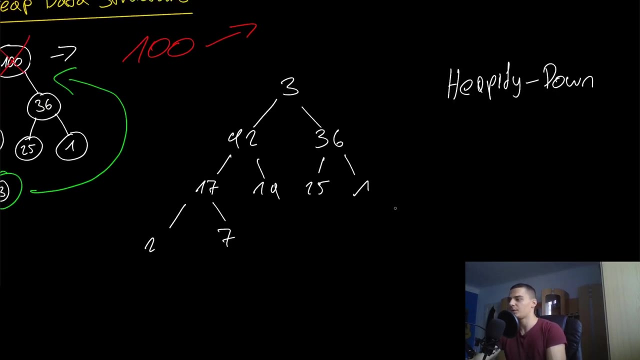 a very small one of the smallest elements is at the root, uh, at the root node. so what we want to do now is we want to uh perform a so-called heapify down. so this is the the opposite of the heapify up operation, the heapify down operation, and what we do here is we just take this element. 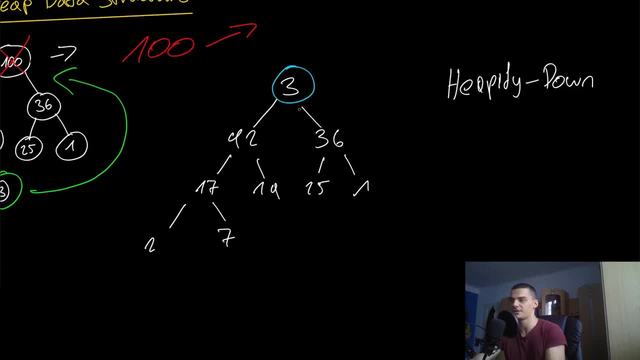 here this root element and we compare it to the largest of its children. so in this case, 92, because, uh, and we compare it to 92, and if 92 is larger than 3 we're going to swap positions. so in this case it is, and because of that we're going to swap the positions of 92 and 3, and 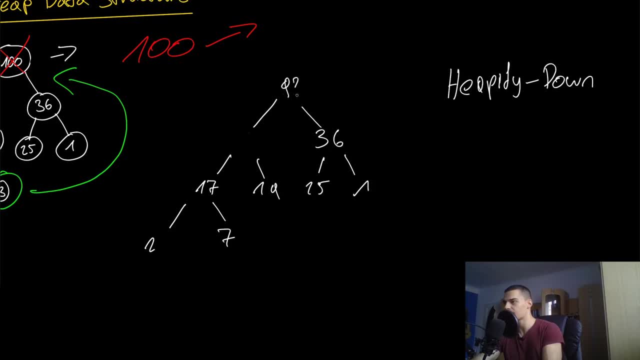 we will get one level down. so 92 and 3. and now you can see why we picked the larger element, because if i was to swap it with 36- which would also be fine, because 36 is larger than 3- uh, we would have 36 as a root node here, which is above 92, even though it's smaller than 92. so you, 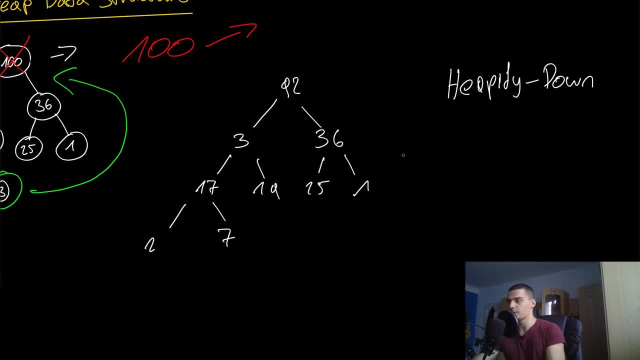 always want to swap it with a larger element or compare it with a larger element to the larger element. now, in this case again, we have the 3 here and we compare it to 19, because 19 is larger than 17. we can see 3 is less than 19. so what we do again is we swap their positions and we say 19 and 3. 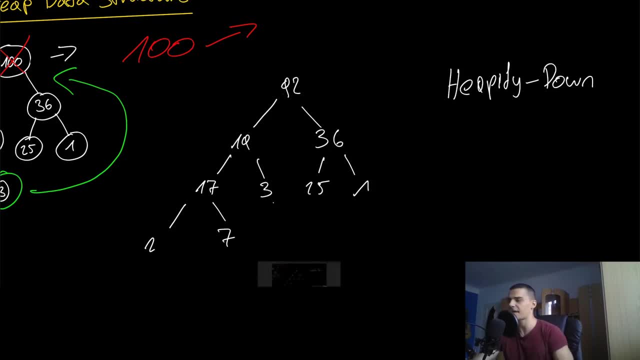 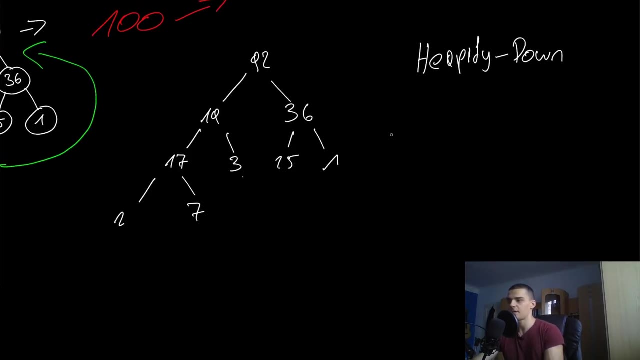 change places. so we have 19 up here and 3 down here and, as you can see, in logarithmic time- same logic as with inserting or heapify up in logarithmic time- we have restored the heap property. we were again satisfying the heap property here, um, and this can be done in logarithmic time. 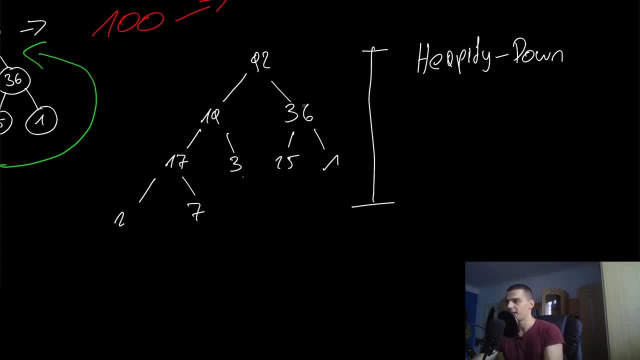 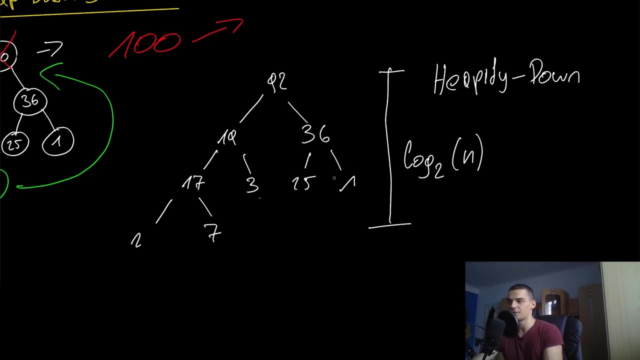 again because we have a logarithmic amount of levels. we have um log 2, a maximum of log 2, um log base: 2 of the amount of elements levels. this is the amount of levels that we can have for the maximum and because of that, the amount of operations that we need to do is logarithmic and thus 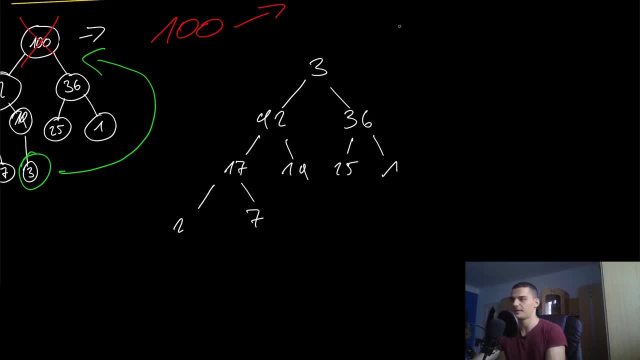 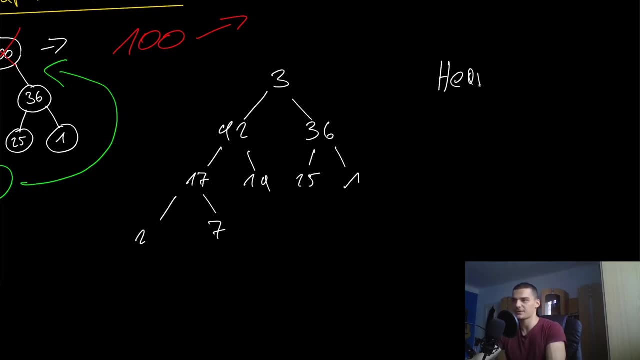 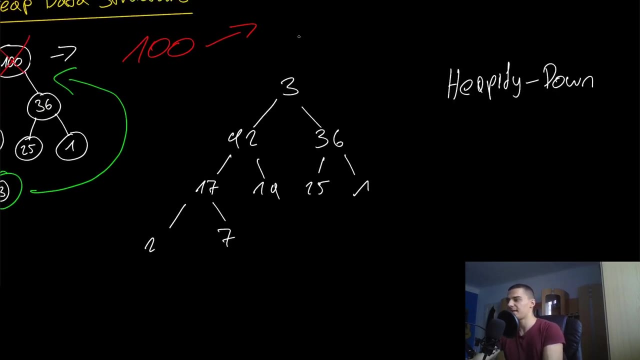 one of the smallest elements is at the root, uh, at the root node. so what we want to do now is we want to uh perform a so-called heapify down. so this is the the opposite of the heapify up operation, the heapify down operation, and what we do here is we just take this element here, this root element. 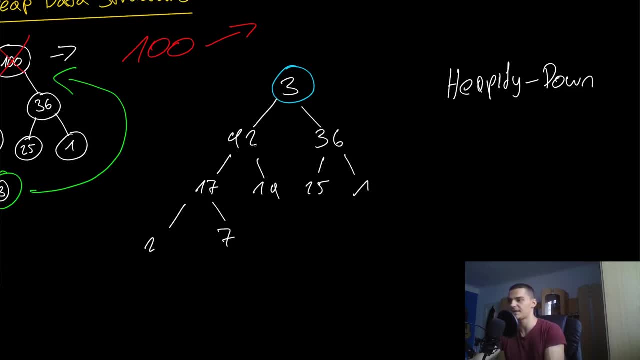 and we compare it to the larger element and we compare it to the larger element and we compare it to the largest of its children. so in this case, 92, because 92 is larger than 36, uh, and we compare it to 92 and if 92 is larger than 3, we're going to swap positions. so in this case it is, and because 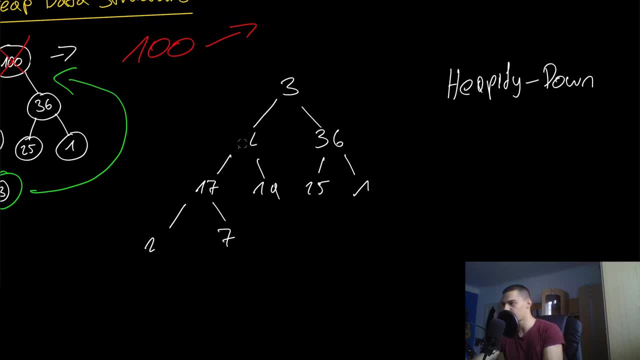 of that, we're going to swap the positions of 92 and 3 and we will get one level down. so 92 and 3. and now you can see why we pick the larger element. because if i was to swap it with 36, and we're going to swap the positions of 92 and 3 and we're going to swap the positions of 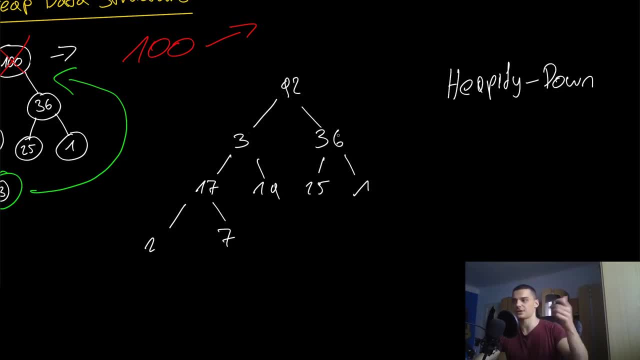 96, which would also be fine, because 36 is larger than 3. uh, we would have 36 as a root node here, which is above 92, even though it's uh smaller than 92. so you always want to swap it with a larger element or compare it with the larger element to the larger element. now, in this case, again, we have 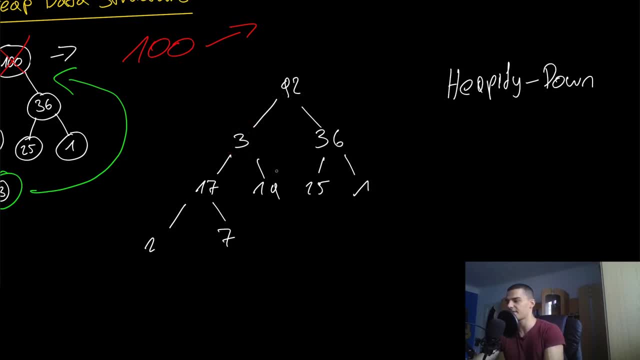 the 3 here and we compare it to 19. because 19 is larger than 17, we can see 3 is less than 19. so what we do again is we swap their positions and we say 19 and 3 change places. so we have 19 up here and 3 down here and, as you can see in logarithmic time, 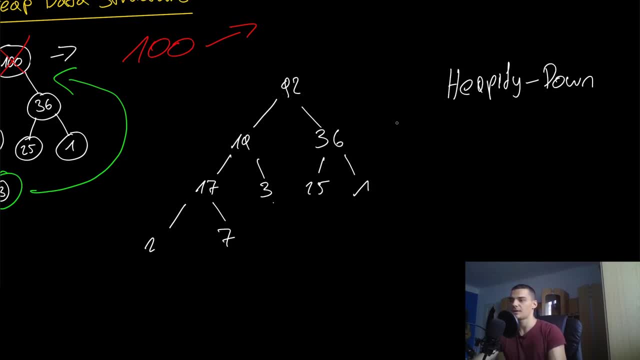 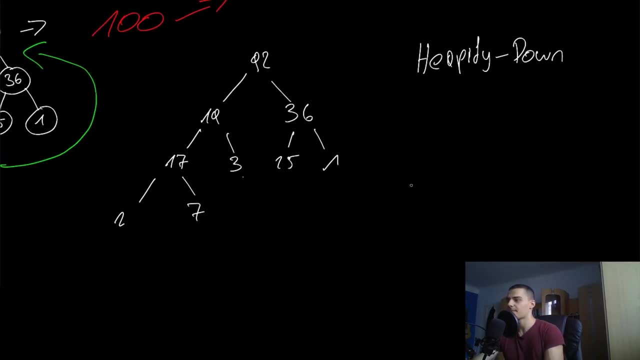 same logic as with inserting or heapify up in logarithmic time. we have restored the heap property. we were again satisfying the heap property here, um, and this can be done in logarithmic time again because we have a logarithmic amount of levels. we have um log 2, a maximum of log 2 um. 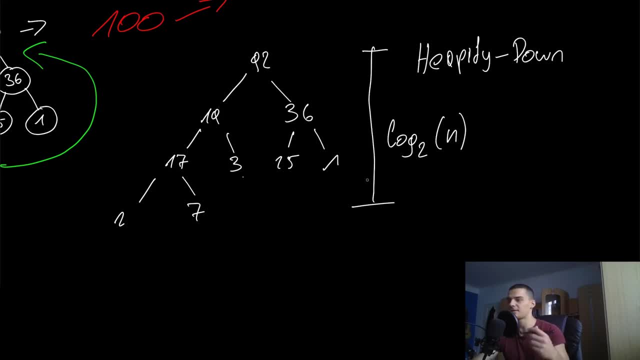 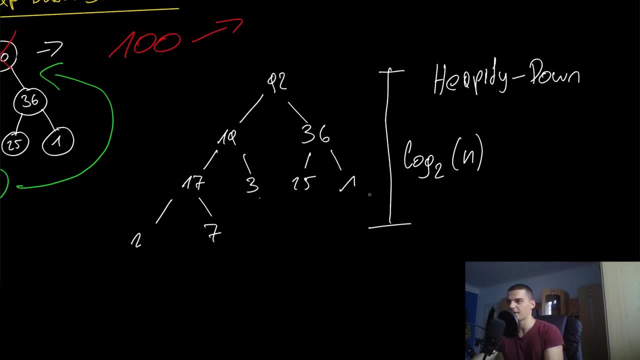 log base 2 um and we have a maximum of log base 2 um and we have a maximum of log base 2 um and we have a maximum of the amount of elements levels. this is the amount of levels that we can have, the maximum, and because of that, the amount of operations that we need to do is logarithmic.